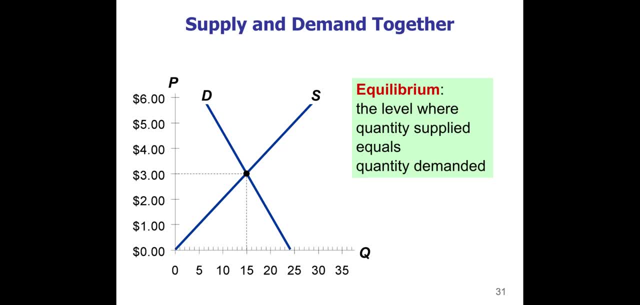 say hello to the other first consumer. You know that. listen long enough to that. but that's not really the case. If we, for instance, want to adjust the quantity wise, what do we do? We call that the equilibrium site. We can add основative values in here. In short, there are 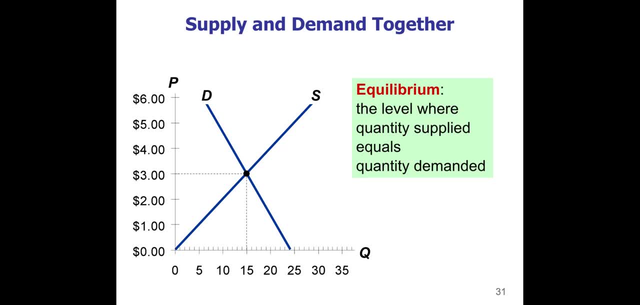 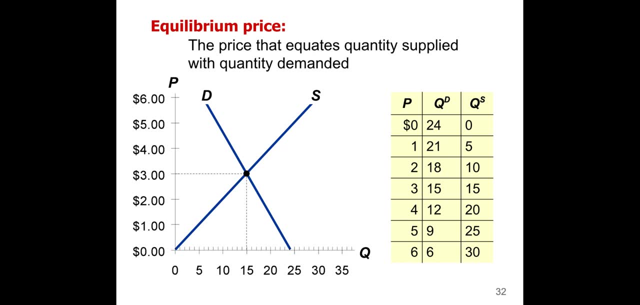 two or more l's here, where the word and 40 to 50 dealers- and the number of dealers will be between the two- should be made. The supplier is willing to produce the product at that price and sell it to you, and you are willing to buy it. Now the equilibrium price just becomes where the demand and supply. 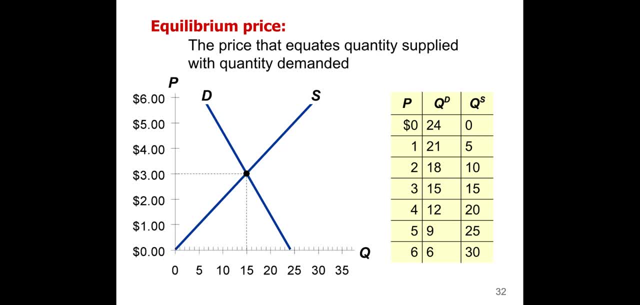 meet. You can also look at the same information on a chart. So this yellow chart here to the right shows you the quantity demanded and quantity supplied at various prices. And you can look down that chart and see that quantity demand and quantity supply at 15 units equal a price of three. 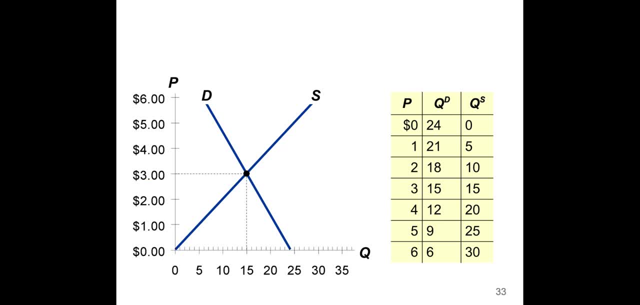 dollars. So that would be our equilibrium. Now the equilibrium quantity is both the amount bought and the amount produced, So the only part of this particular graph that matters is where supply and demand meet. The rest of these lines are theoretical options as to what suppliers would like to do if 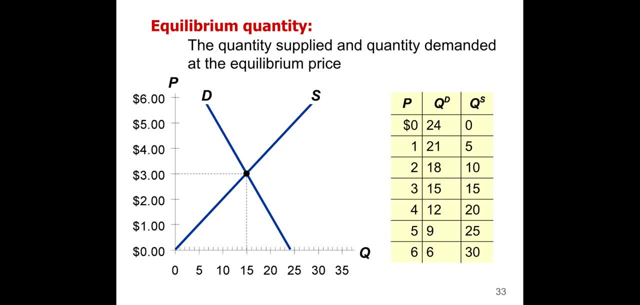 or what buyers would like to do if. So, the only part of this particular graph that matters is what suppliers would like to do if. But the only place that matters is where the supply and demand meet, and that is the equilibrium price and the equilibrium quantity. Now, this is the genius of 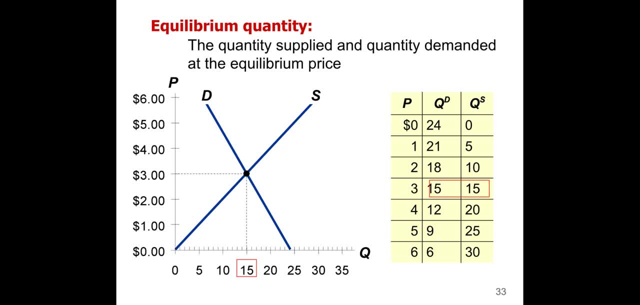 markets, because if the supply and demand- in this case, if they didn't make 15 units and they price them at three dollars, they will sell all 15 units because buyers are willing and able to purchase this product at three dollars and then they would be making profit. But something 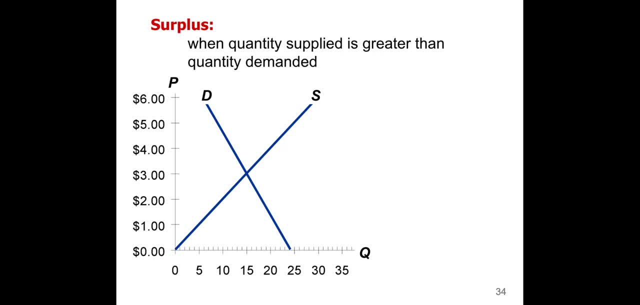 else happens. A surplus can also happen, and this is when quantity supplied is greater than quantity demanded. So let's say that one particular supplier or multiple suppliers in a market get really greedy and they don't want to sell their product for three dollars, They'd rather sell their. 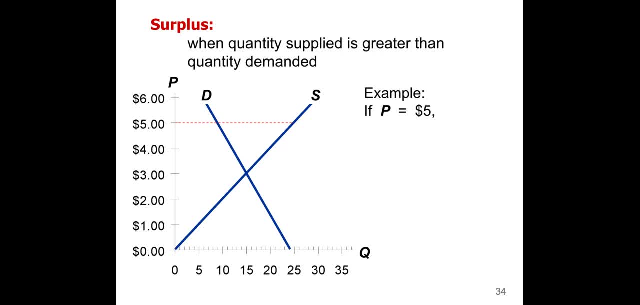 product at five dollars. Well, the problem with that: if you take this five dollar line and walk it across the five dollar line, quantity demanded and quantity supplied are different. The amount of buyers that want to buy a product at five dollars is going to be different. So the amount of buyers that want to buy a product at 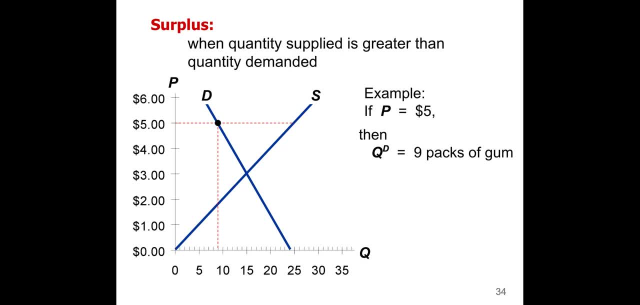 five dollars is only nine people. But suppliers, thinking that they were going to make tons and tons of profit on these packs of gum, then supplied 25 units. Remember, the supplier has to pre-produce the units before they come to the buyers. So now we have a surplus in this particular case, because 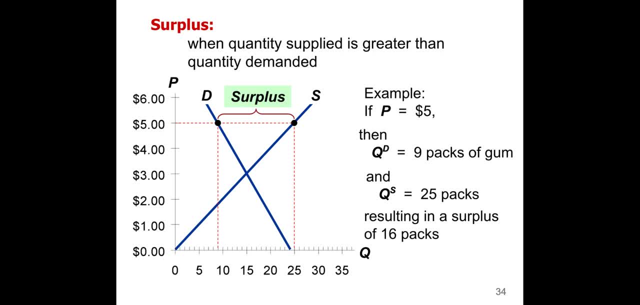 we have numbers on our graph, We can calculate that we have a surplus of 16 packs of gum, And these are packs of gum priced at five dollars that nobody else wants to buy. So if you have a bunch of units that nobody wants to buy, what do you do with them? 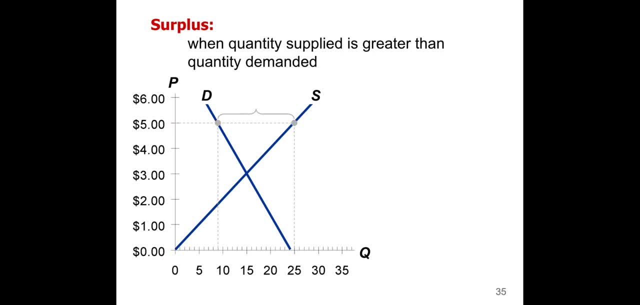 You put them on sale. So in the free market the seller is going to lower the price, and when they lower the price to four dollars we've got more people- that's quantity demanded- that are willing to buy the product and they purchase them. So your supply or quantity supplied is going down. 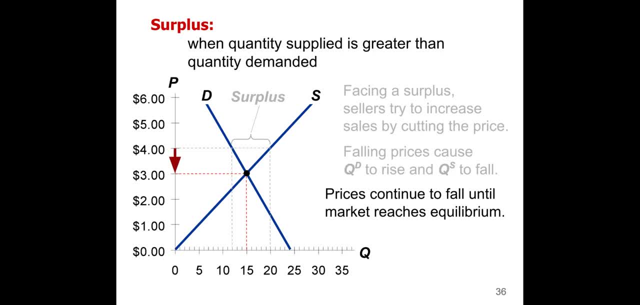 And this is a good example for that. If you have an existing product, if you're selling out of one of those products, you're going to lower the price to five dollars And then you go to the place that it's supposed to be, for example, selling all of the products that are in the 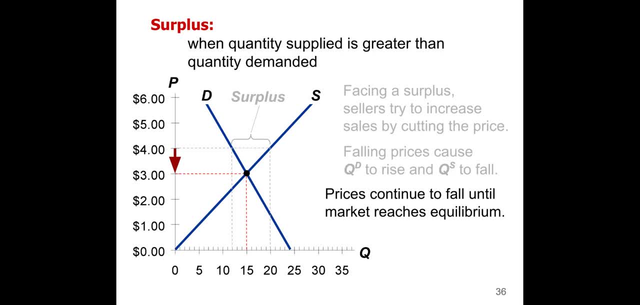 free market. So everybody in the free market is going to have to go back into the market and they're going to have to go back and the next day we have the sales proposal that we're going to have at the end of the year. So we're going to have a big subcontractor in the market to buy a single product and then we're going to have a big sale in the month of May. 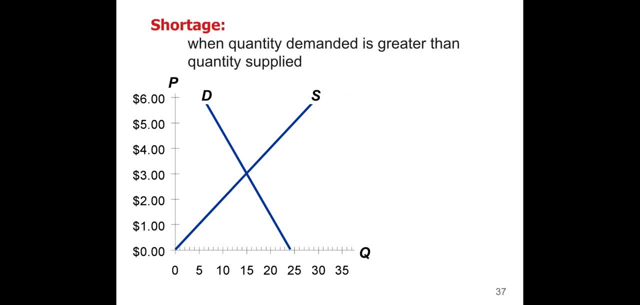 goods. Now, of course, the opposite could happen as well, and we call this a shortage. A shortage is when you have quantity demanded that's higher than quantity supplied, and that's caused when you price the product too low compared to what the market wants, So at a price of $1,. if you follow that red line, the 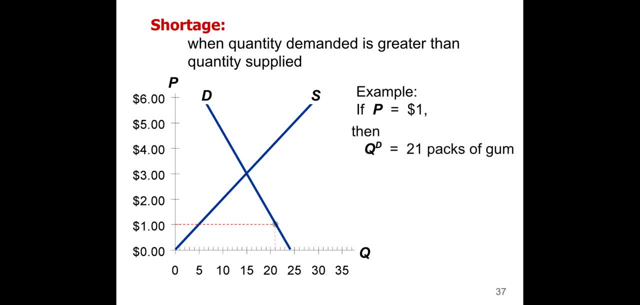 quantity that the gum manufacturer supplied was really low. because their profit margin is so little it might not be worth it to them, But at a price of $1, lots of people want to buy packs of gum. So quantity demanded is 21.. Now if